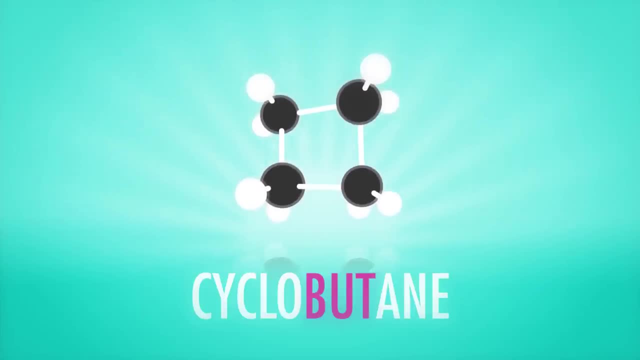 Cyclobutane, with its four carbon atoms, is still fairly unstable and reactive, while in cyclopentane the bonds are even more stable because they form something close to those tetrahedral bond angles, While the bond angles in cyclohexane are basically perfect for the tetrahedral orbitals to overlap without strain. 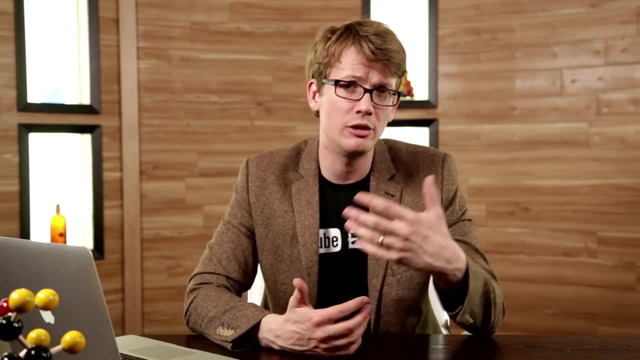 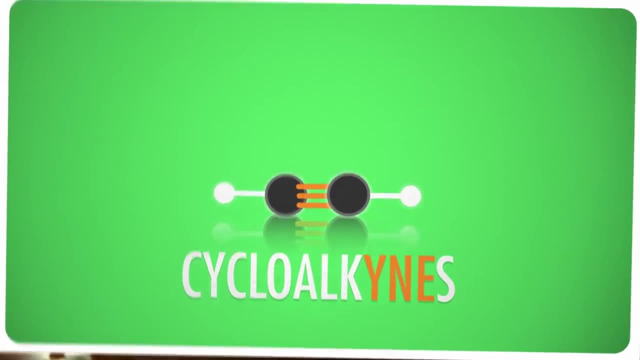 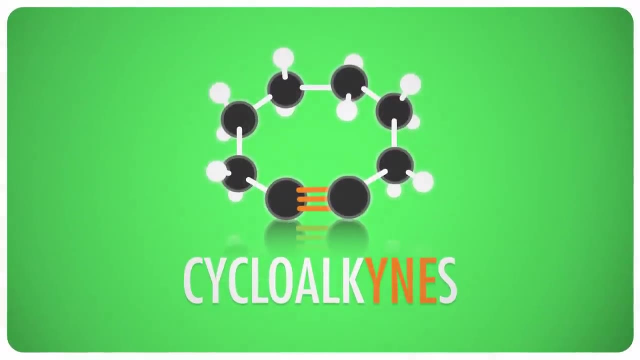 Cycloalkenes also start at three carbons and get increasingly stable as more are added, though their double bonds make their molecules planar instead of tetrahedral. Finally, cycloalkynes do exist, But they are crazy hard to form because the triple bond is linear, so it hates bending into rings, and that is why the simplest cycloalkyne has eight carbons. 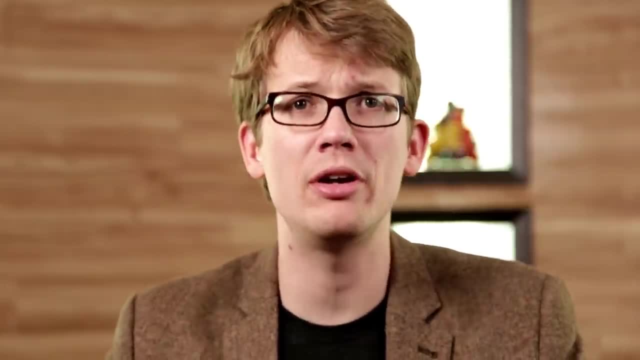 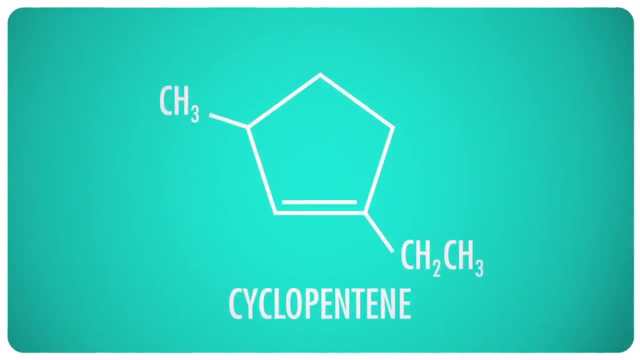 Of course, these rings can have all sorts of things stringing off of them, and their names work almost exactly the same way as straight chains do. this ring has five carbon atoms in a double bond, so it's a cyclopentene. 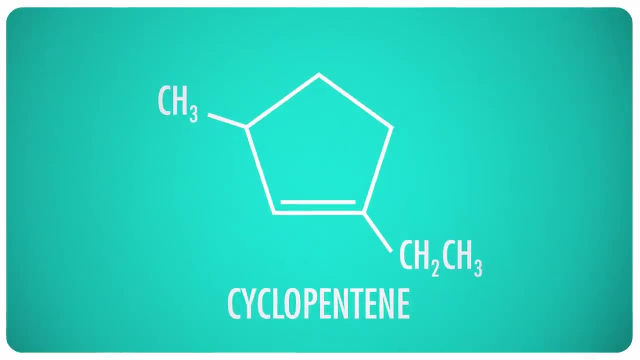 It has two branches, an ethyl group and an methyl group. We list these in alphabetical order in the name And we number the carbons in the ring so that we get the lowest possible numbers on the branches And on the double bond. 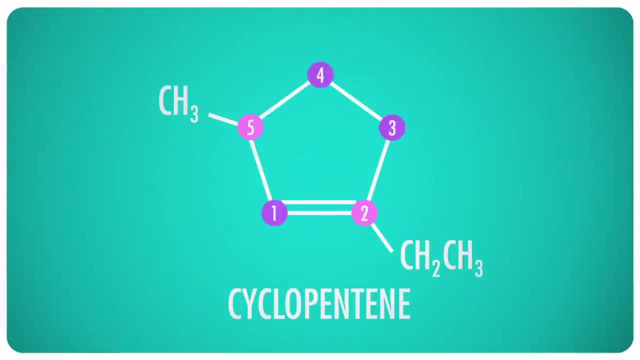 If we number counterclockwise from the beginning of the double bond, we get the branches at the two and five positions. But if we number clockwise from the double bond, the branches are at the one and three positions. So this must be 1-ethyl-3-methyl-cyclopent-1-ene. 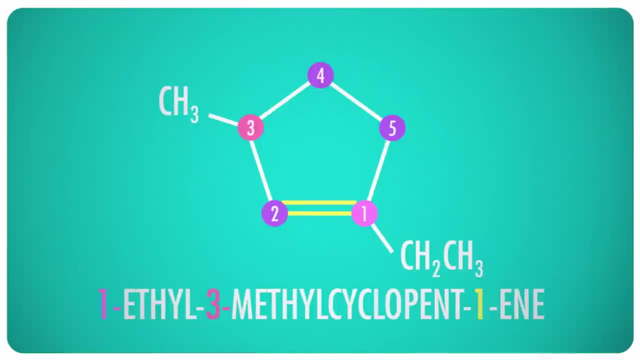 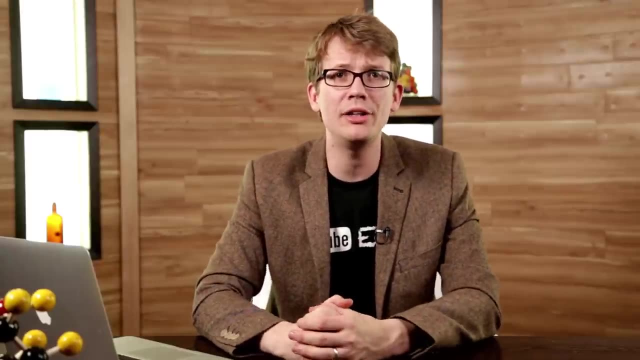 But since there's only one double bond and it's in the first position, the second one is often left out as being understood. So we simply call it 1-ethyl-3-methyl-cyclopentene. Incidentally, all of the identifying parts of an organic molecule- the double and triple bonds, the carbon chains that branch off the main chain, 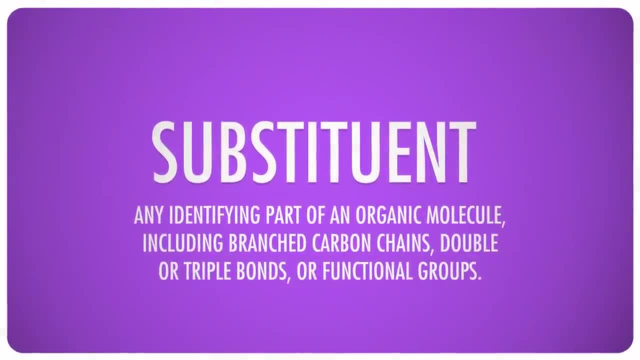 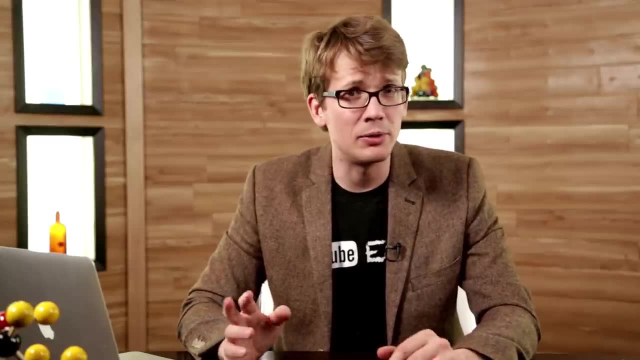 those are called substituents because they substitute for hydrogen atoms, Or we've just been looking at the cyclic hydrocarbons. So what's up with the aromatics? How are they different? Well, this is one of those times when carbon starts doing some of its spectacular dances. 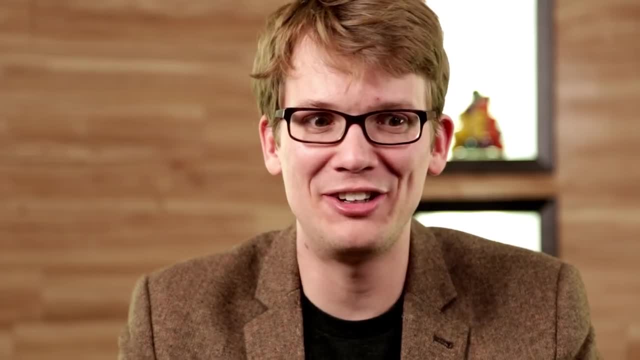 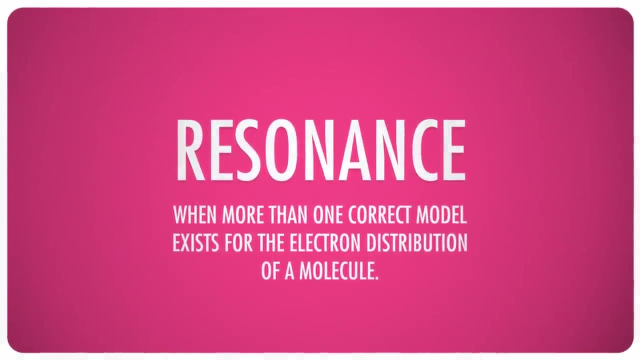 Cyclic hydrocarbons that contain resonance structures. Things are getting interesting, And by interesting I mean what Resonance occurs when electrons are distributed around the molecule in a way that makes it impossible to draw with a single Lewis structure. It's a limitation of our tools to represent the beauty in carbon. 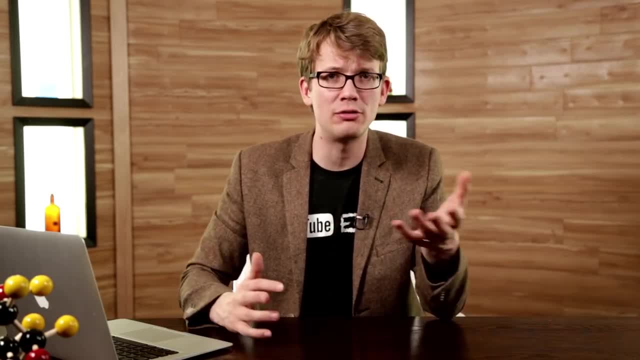 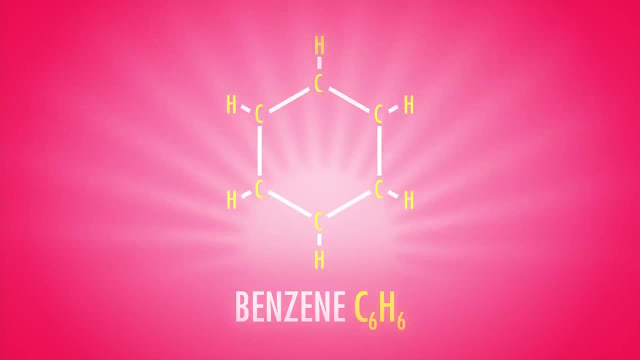 And complexity of reality In a resonance structure. the real world structure of a molecule is essentially an average of all of the possible structures that we can draw. The simplest aromatic hydrocarbon, and one of the most common is benzene- C6H6.. 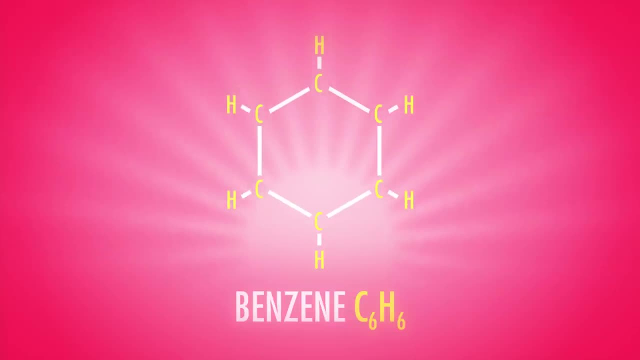 It's the pungent compound that gives gasoline its strong sweet smell. It contains three double bonds, so that each carbon has a total of four bonds. We normally write this and other organic structures without the hydrogens in order to simplify things, And we often don't even write the C's for the carbons. 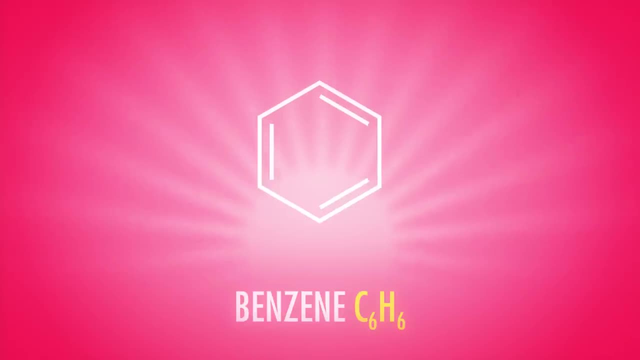 Every corner is assumed to be a carbon atom, And since we know that carbon needs four bonds, it's easy to figure out where the hydrogens belong, even when they're not written. Here's the thing, though: Those double bonds could just as easily be in these positions. 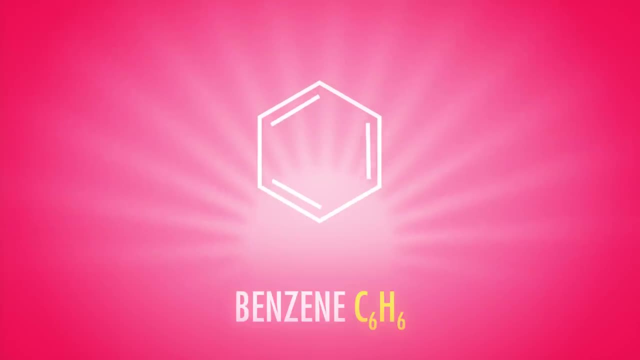 And they are in those positions, Sort of Remember. there are two types of bonds in double bonds. There's those sigma bonds that happen linearly, And then there's those p orbitals that stick up above and below the plane of the molecule. 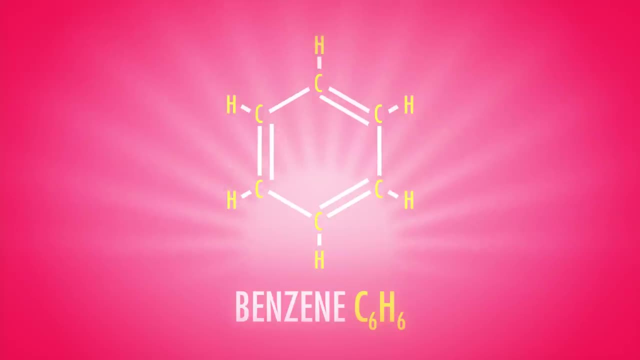 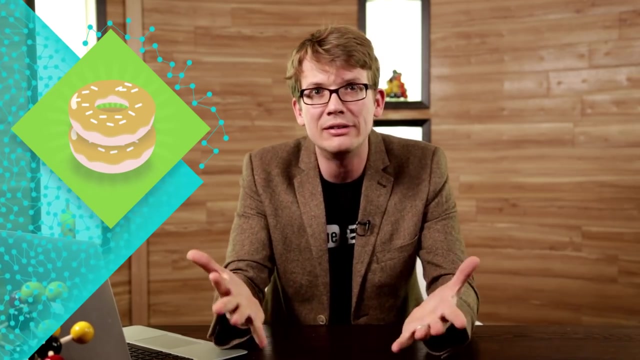 Those p orbitals in an aromatic compound all merge together in a ring that stretches above and below the whole molecule. It's a distribution of electrons that's like a doughnut. It's extremely stable. Overall the bonds are in both places. so the actual structure is essentially an average of the two drawable Lewis structures. 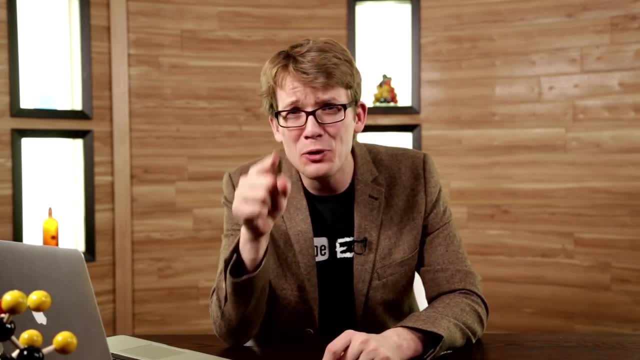 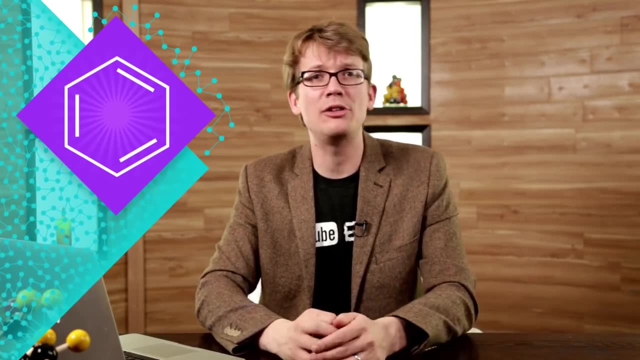 That's resonance, It's reality, poking us in the nose and saying: Oh, you thought you were so clever with your Lewis structures, but in this situation they are useless. To show that the double bonds aren't in any specific place, we often just show the structure with the circle in the middle. 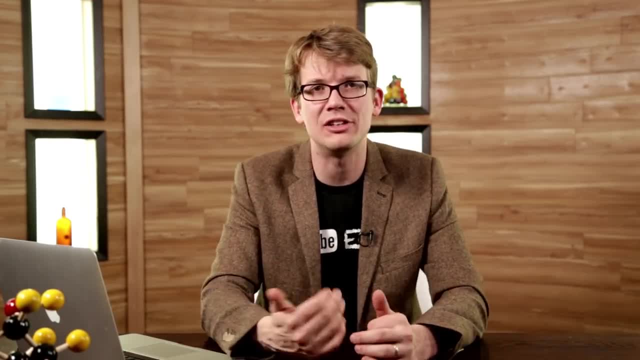 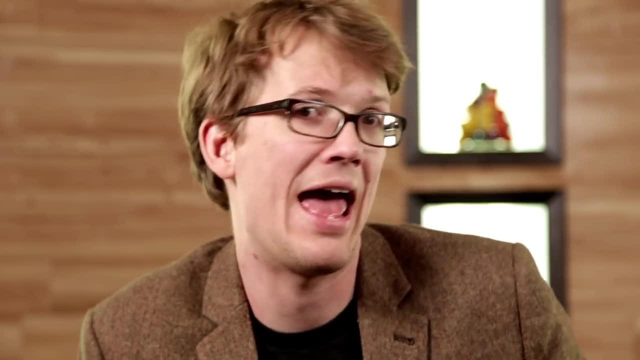 signifying that the double bonds are averaged in a ring throughout the benzene group. Technically, the number of bonds between each pair of carbons is defined as 1.5.. It's not a double bond, it's a one-and-a-half bond. 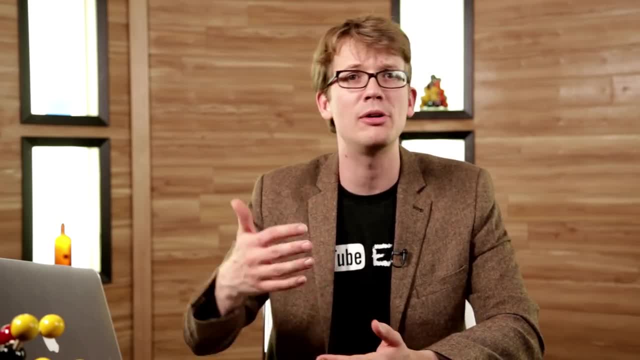 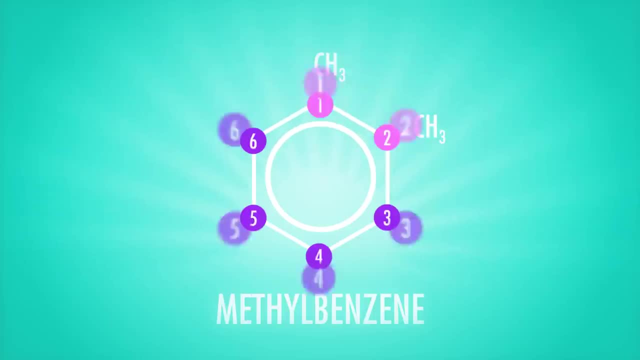 Now, aromatics can have all sorts of substituents as well, and the naming system is pretty much the same as with other cyclics. Another example: So this is a benzene with two methyl groups on it. As always, we number the rings so the branches have the smallest possible numbers. 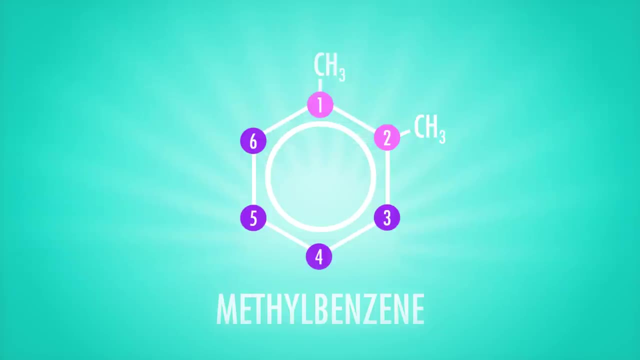 In this case, if one of the methyl groups is in the one position, the other is in position two. Note that the numbering could also be done like this, but it doesn't matter as long as the branches are at the lowest possible numbers. 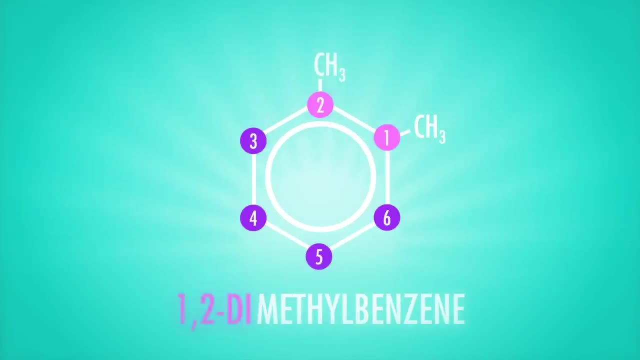 That makes this molecule 1,2-dimethylbenzene. Now if you swap the methyls out for a couple of other slightly more complicated numbers, you'll see that the numbering is the same as with other cyclics. Now if you swap the methyls out for a couple of other slightly more complicated groups, then you get acetylsalicylic acid or aspirin. 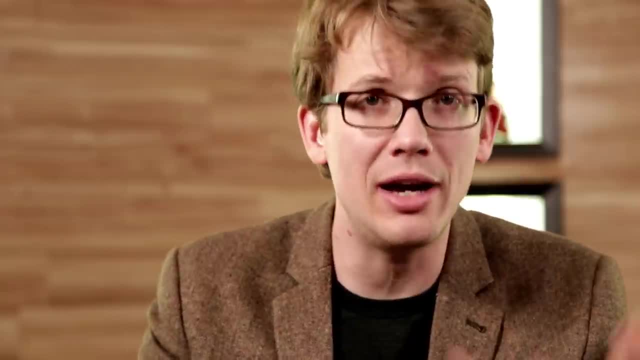 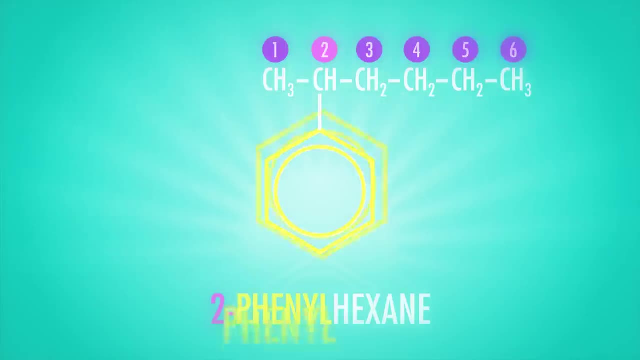 Aromatic rings can be used the other way around too, as substituents onto hydrocarbons. Check out this molecule: a hexane with a benzene ring attached to carbon number two. When benzene is used as an attachment, we call it a phenyl or phenyl group. so this is 2-phenylhexane or 2-phenylhexane. 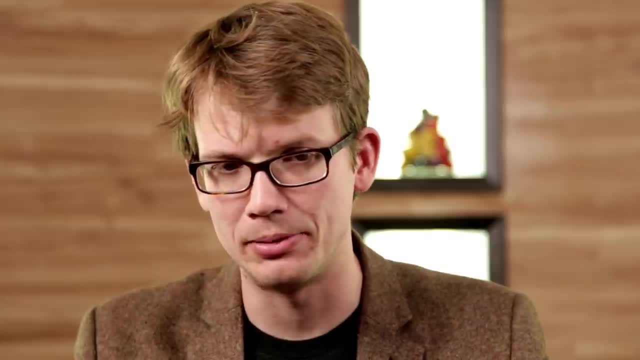 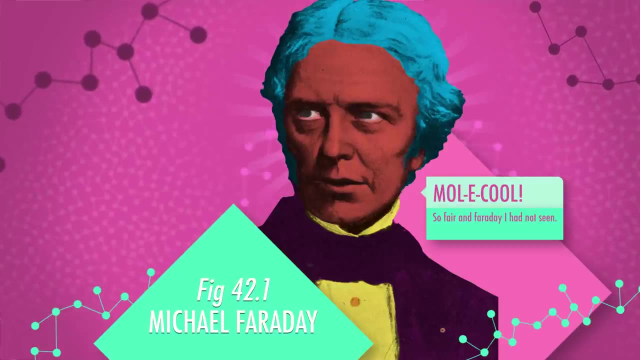 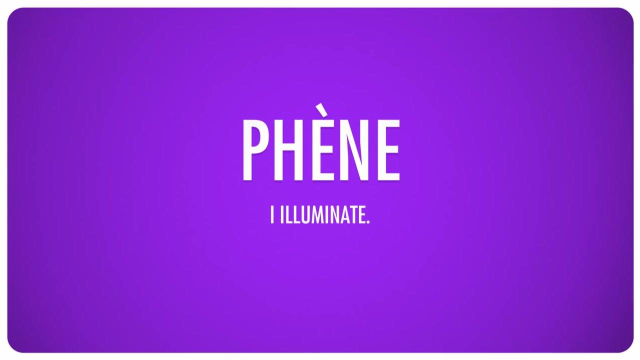 It doesn't matter. What's important is that it is not a benzyl group. Why, Well, it was English genius Michael Faraday who first isolated benzene. He extracted benzene in 1825 from the gas used in lamps and in honor of this, his French contemporary chemist, Auguste Laurent, started calling the derivatives of benzene phen from the Greek for I illuminate. 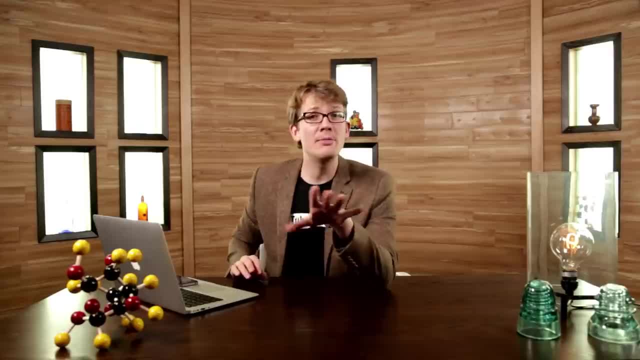 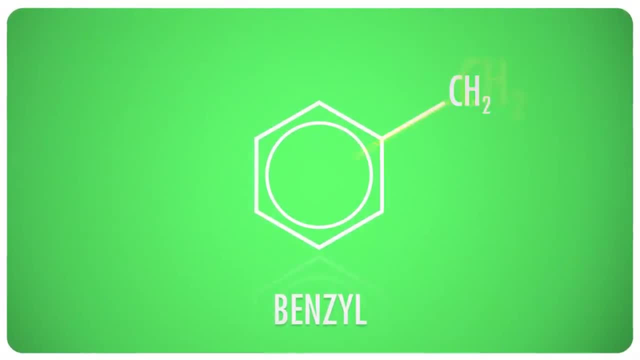 It's a lovely gesture, very sweet, but like, seriously, But just to make sure you're like good and solidly confused, benzyl groups do exist. They're a phenyl group joined by a methyl group instead of just directly. 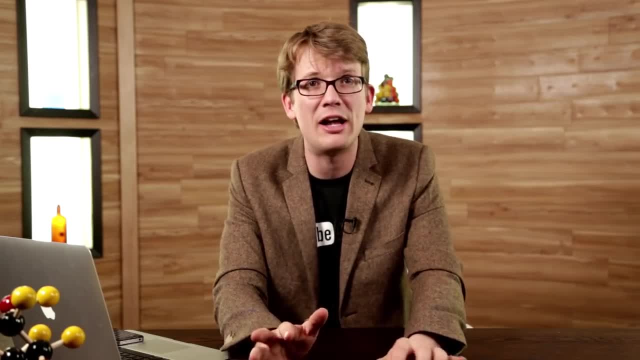 So, now that we know where the word phenyl comes from, I bet you're just salivating with curiosity, wanting to know where benzene comes from, Because, like you're desired to know Things is stronger than any of your other desires, right? 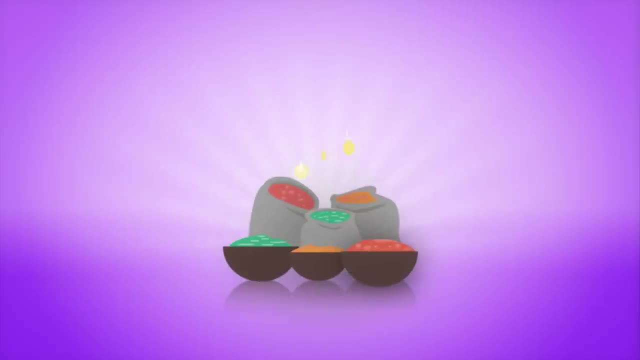 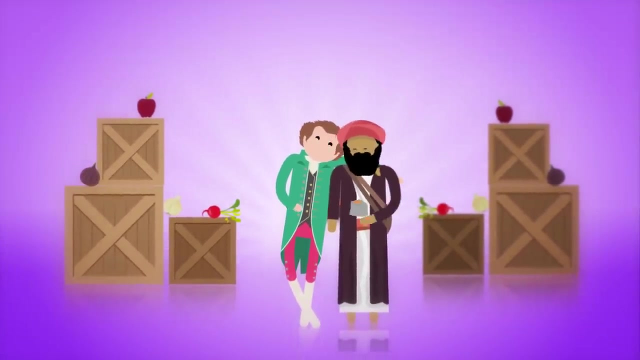 Yeah, I thought so. So here's how it happened. Back in the 1400s, when the spice trade drove the majority of the global economy, Arabic traders sold European traders a resin used in perfumes and medicine that they called lubanjawi, or incense of Java. 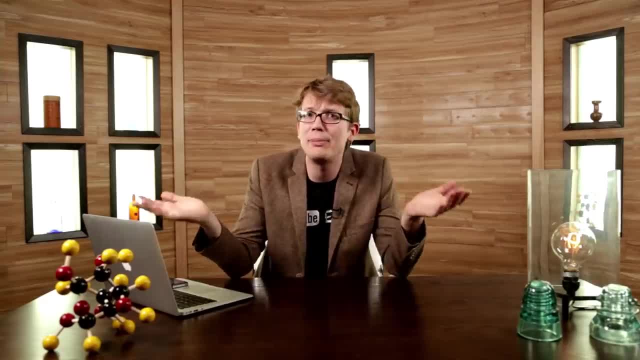 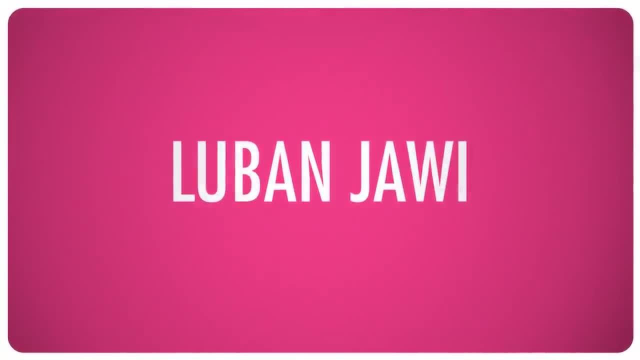 Of course it didn't come from Java, it came from Sumatra, but the world was a big and complicated place, so we can't really blame them for being a little bit confused. The lube was mistaken by the Italians for the definite article la, and so it was dropped, making it banjawa. 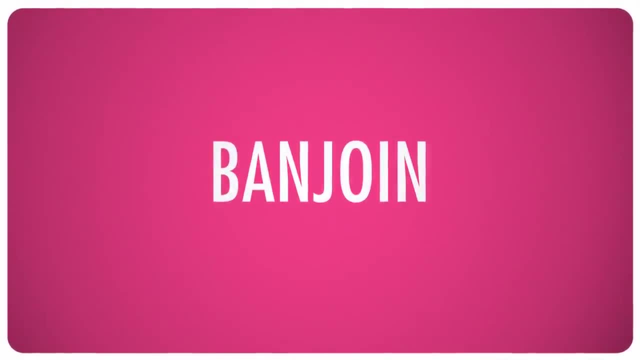 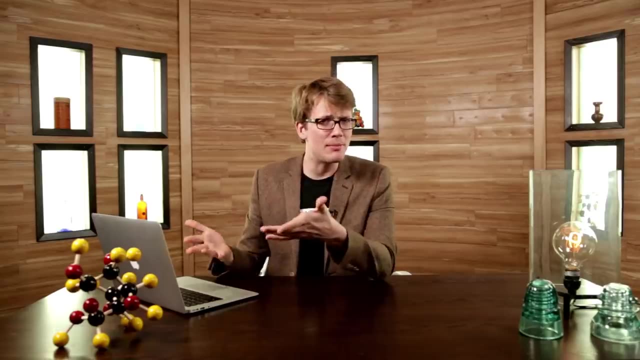 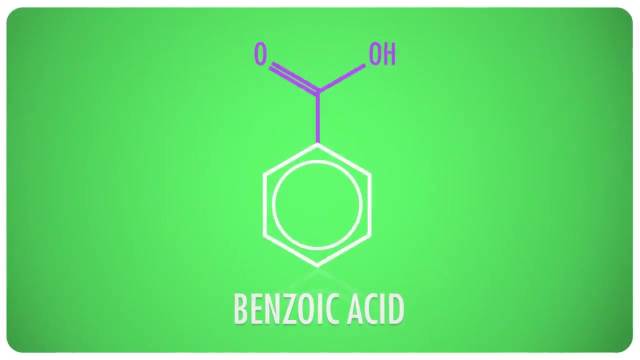 And then the French called it banjwa and eventually the German and English made it benzoin. This is also, by the way, the same root as the name Bon Jovi, it's not. When we started doing some chemistry, we found that most of benzoin was composed of an acid which chemists named benzoic acid or acid of benzoin. 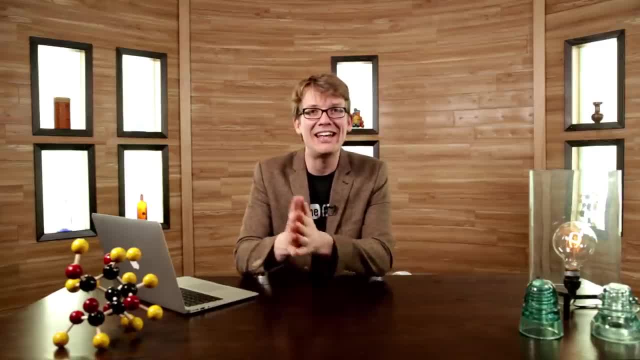 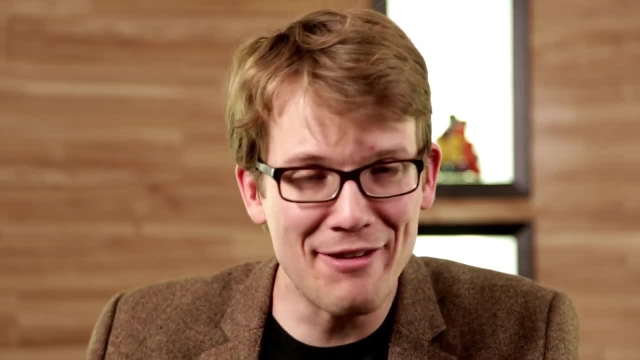 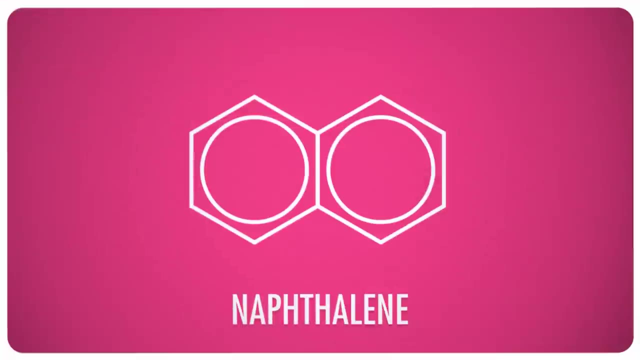 Then a little chemistry knocked the acid off, creating what was clearly an alkene. so they named it benzene, because it was an alkene that was from the benzoin resin. History is hiding everywhere, and so is chemistry. Now benzoic acid is one of literally infinite possible benzene-based compounds. 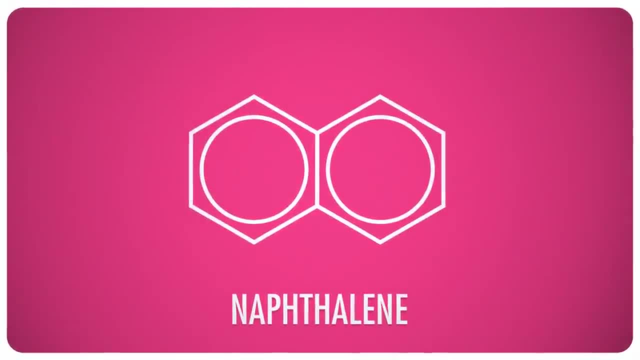 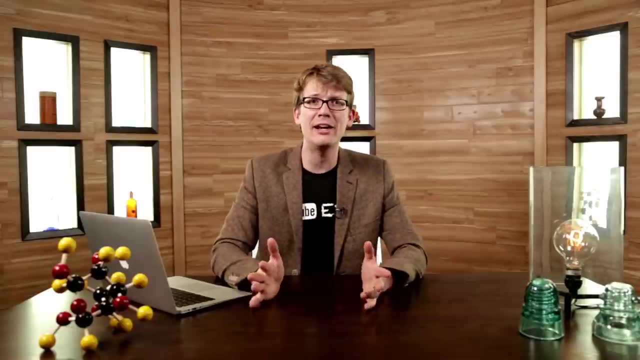 There's naphthalene, the main ingredient in mothballs. it's basically two benzene rings stuck together. Then there's anthracene with three benzenes, which is probably the dye that's making your blue jeans blue, and it can get crazy complicated all the way up to humic acid, a component of soil. 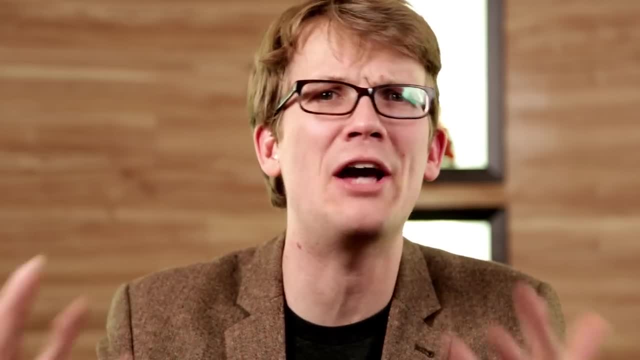 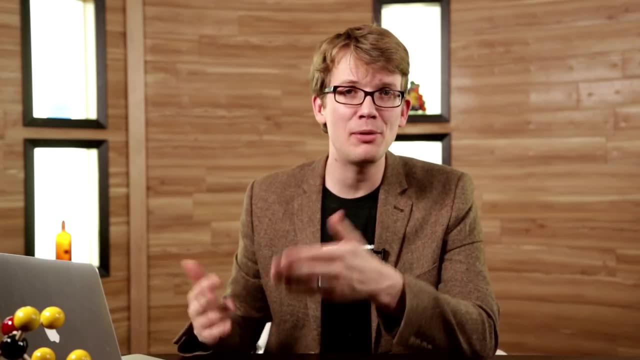 Now you might be wondering how something so complicated as that could ever even come into being. Like any organic compound, aromatics can undergo tons of reactions that produce all sorts of molecules. By far the simplest and most common are substitution reactions, In which one substituent is substituted for another. Like one of the hydrogen atoms on a benzene might be changed to a propyl group, or then a halogen might come in and replace that propyl group with a bromine. These changes alter the compound, of course, but it may not be that major a change like changing your shoes, unless you put on some really weird shoes. 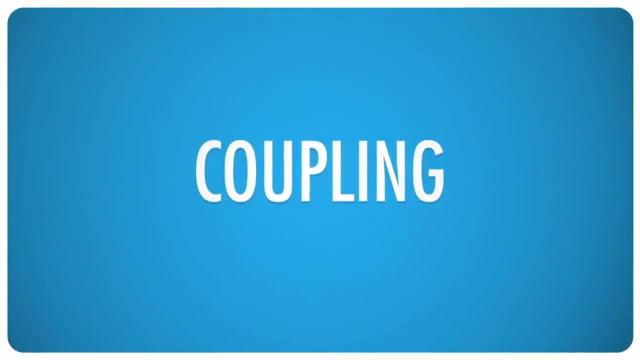 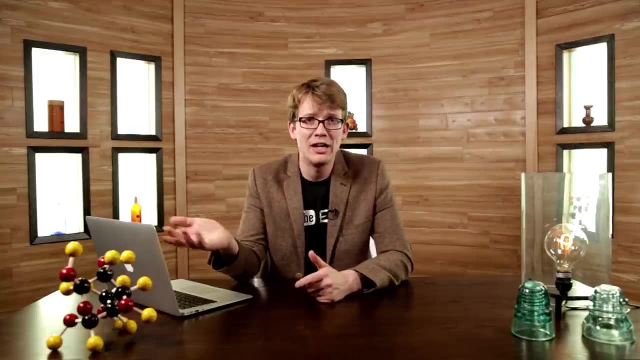 Another fairly common reaction of aromatic hydrocarbons is coupling, the joining of two aromatic structures, And it basically works the same as a substitution reaction. the only difference is that the new substituent is another aromatic structure And it typically requires some kind of a fusion. 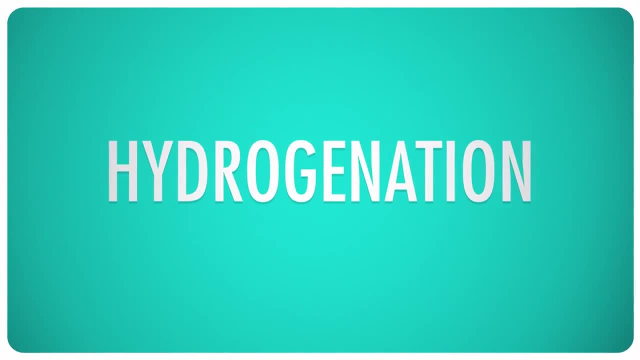 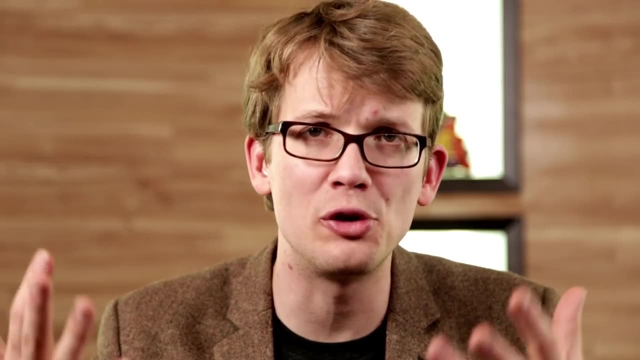 A final common reaction of aromatics is hydrogenation, which we talked about a little last week, the addition of hydrogen atoms to remove double bonds. Now, of course, getting rid of even a single double bond in a phenyl group always destroys the resonance and thus it is no longer an aromatic compound after hydrogenation. 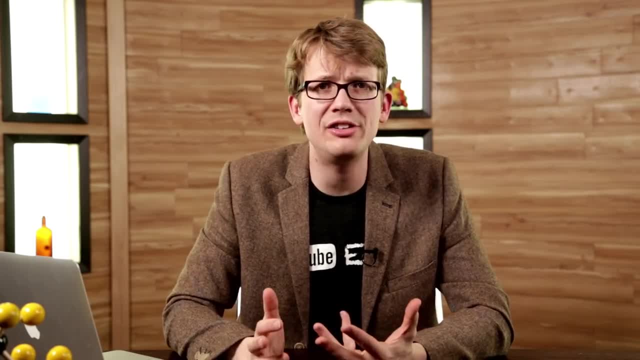 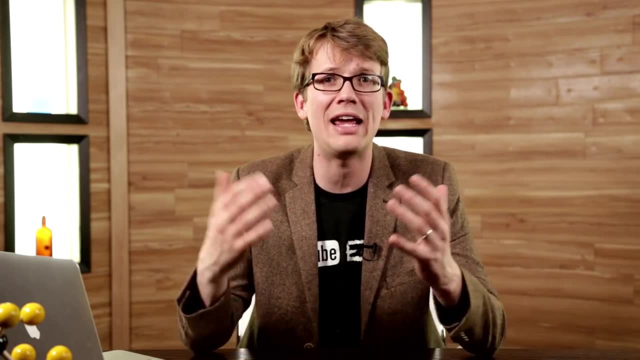 Now, obviously we haven't covered all of the possibilities here, but you can already see that organic molecules have the potential to become extremely large and complex, integrating straight chains, cyclic structures and aromatic groups in the same molecule. This literally infinite variety is what we're looking for. 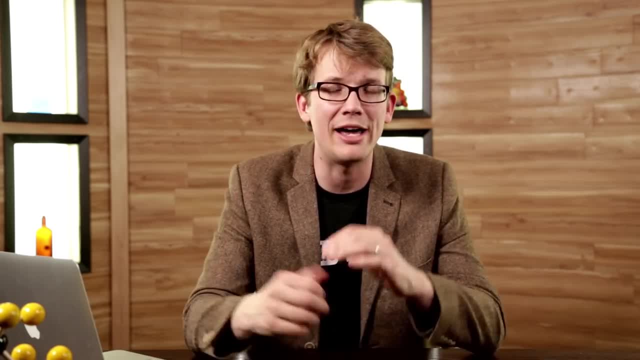 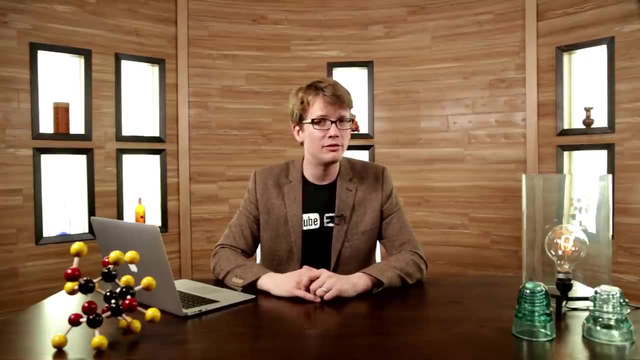 Variety is what makes organic compounds the basis for the infinite variety of life on Earth. So I'll leave you to your genes in basil, pesto and aspirin now to appreciate them on a whole new level. that simply was not possible just ten minutes ago. 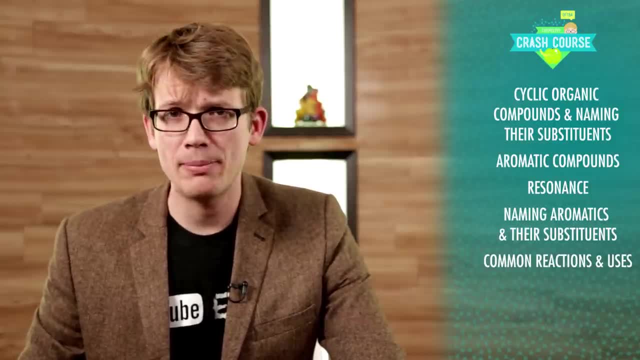 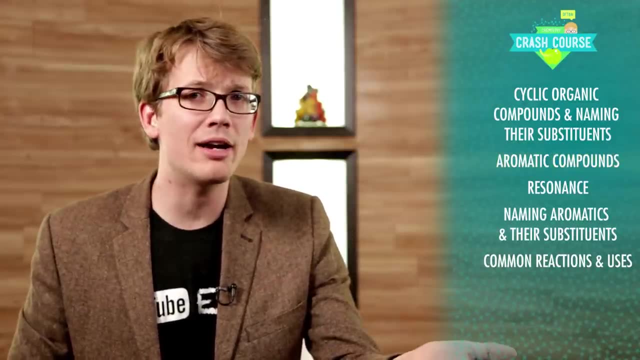 Meanwhile. thank you for watching this episode of Crash Course Chemistry. If you paid attention, you learned about the structure of cyclic organic compounds and how to name them and their substituents. You also learned what an aromatic compound is, what resonance is, and how to name aromatics and their substituents. 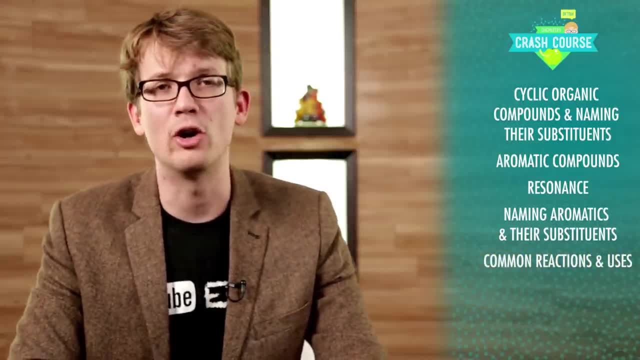 And finally, you learned a few common reasons. You learned about the reactions and uses for aromatic compounds. This episode was written by Edie Gonzalez and myself. it was edited by Blake DePastino and the chemistry consultant was Dr Heiko Langner. 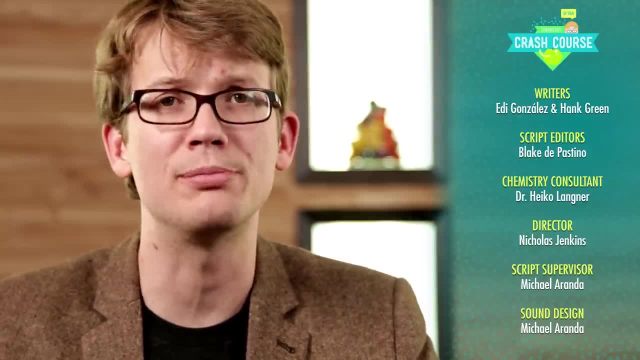 It was filmed, edited and directed by Nicholas Jenkins, the script supervisor was Michael Aranda, who is also our sound designer, and the graphics team is Thought Cafe.